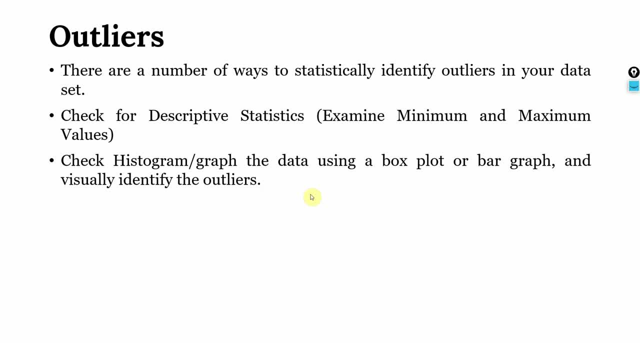 Now check for Histogram graph the data using a Boxplot or Bar graph and visually identify the outliers. To get a map of the various data sources, access to a database should have two sliders: one on the left, one on the right and another shows a bar chart. 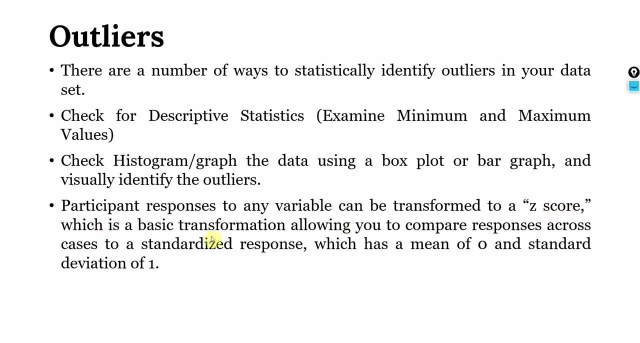 Now POS gera terms can be lovely. Each of the intervals should contain some references related to ones that theemas should follow. Participant responses to any variable can be transformed to a zero orderوع Gaussian variable response z score, which is the basic transformation allowing you to compare responses across. 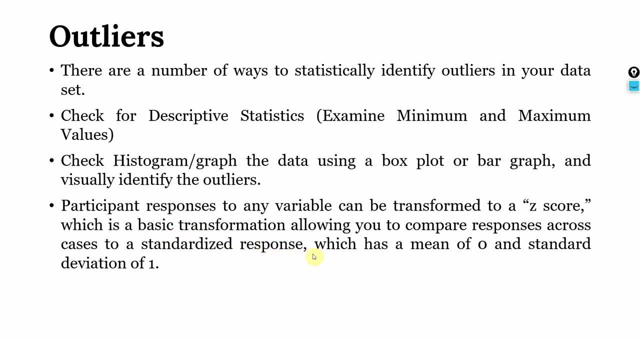 cases to a standardized response which has a mean of zero and a standard deviation of one. so what you can do is you can transform the participants responses to a z score, and that can obviously highlight the outliers as well. and if your z score is greater than 3.3 plus or minus, it can be. 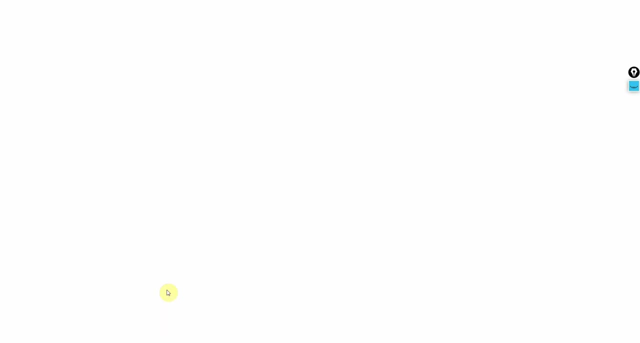 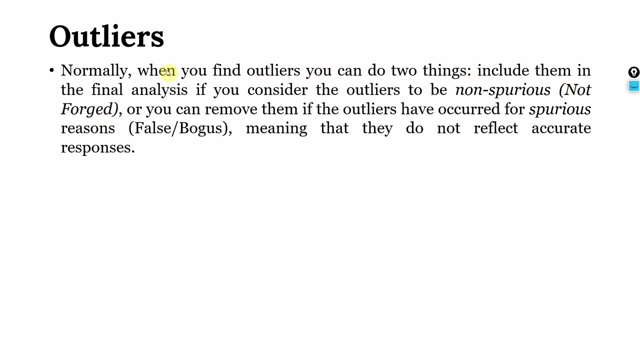 considered as an outlier. now, normally, if you find outliers, you can do two things: include them in your final analysis if you consider them not forged or non-spurious, or you can remove them if the outliers have occurred for false or bogus reasons. now, if the outliers don't make sense in, 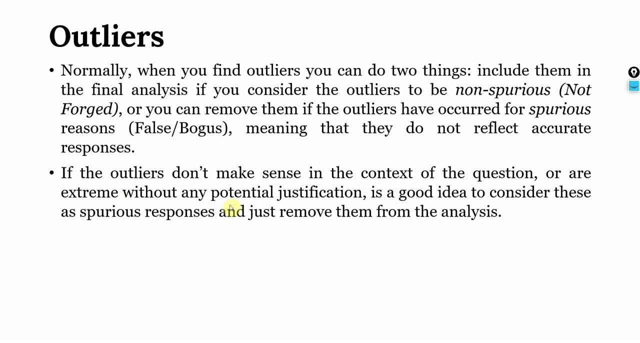 the context of the question or are extreme without any potential justification, it's always a good idea that these responses shall be removed. however, if you find the responses that make sense and are only slightly over the z score of 3.3, then you can keep them. 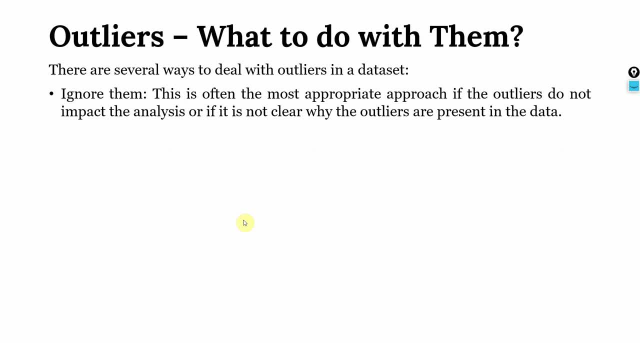 now again, what to do with them. now there are several options. you can ignore them if they are not affecting your responses or your data a great deal. you can trim them. this involves removing the outliers from the data set, and this is just to demonstrate how you can easily go. 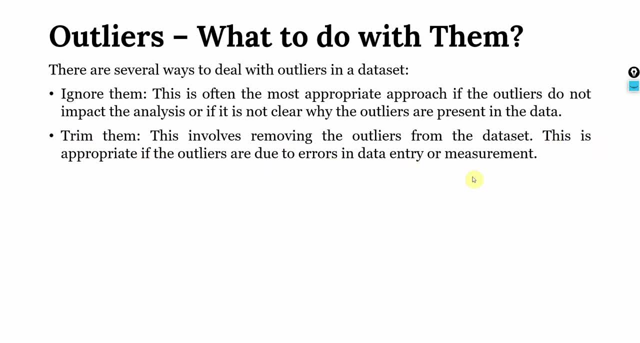 is appropriate if the outliers are due to errors in the data entry measurement. now for this. if you are doing survey based analysis, a good idea is go back to the field questionnaire in hard form or maybe if you have imported them. maybe you have made a mistake while doing something. just double check your. 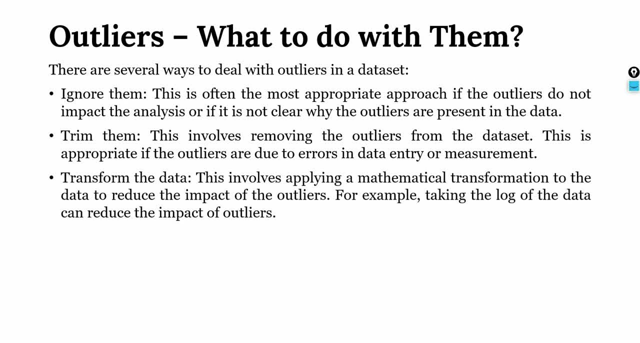 original data now transform the data and this is by taking the log of the data and it can reduce the impact of outliers. so you can do mathematical transformation now. otherwise you can do replacement of the outliers by identifying the fifth and ninth percentile score. so if there is an 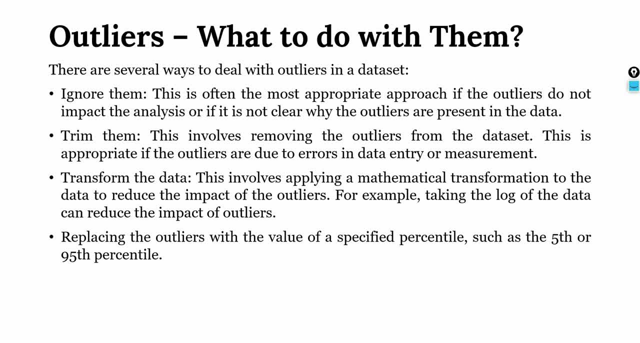 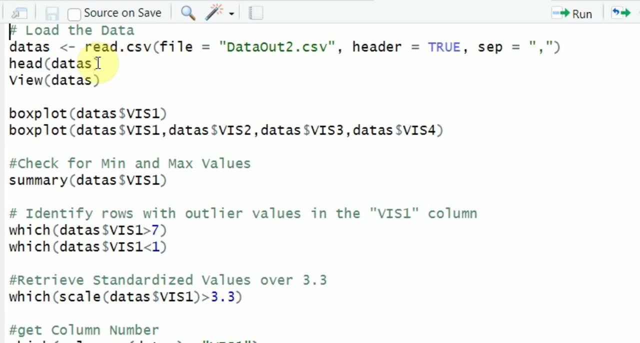 outlier, replace it with a fifth or 95th or 95th percentile score. now it is very important to carefully consider the appropriateness of each approach, as removing or ignoring outliers can sometimes distort the analysis and lead to incorrect conclusions. now, how do we do outliers analysis in R? now again, the first step is to load the 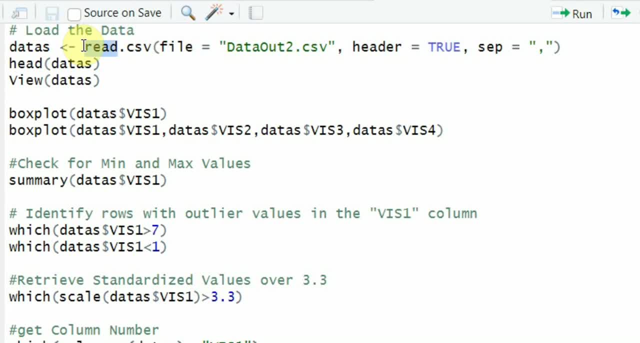 data again whenever you're loading the data. obviously, for now we are using CSV files or Read dot CSV, the file name, and it is in the same folder as I have my R script file. the second argument is: header is, you will, true and the separator is comma. 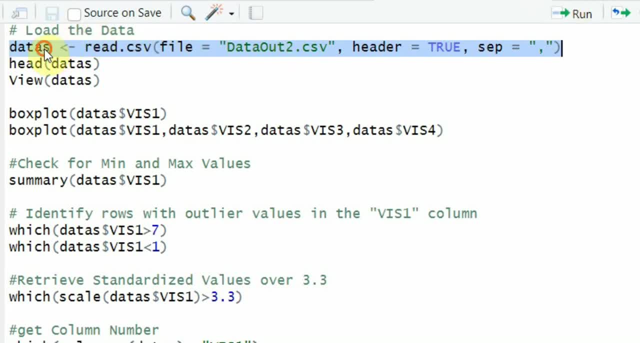 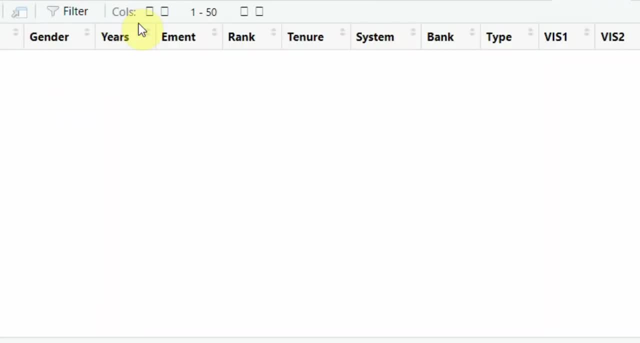 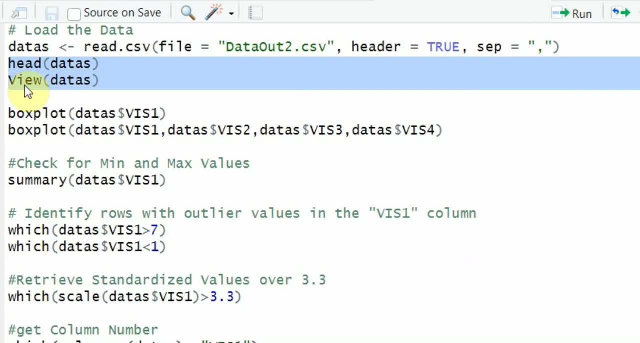 just run it and now you've got data in this object. you want to view it or you want to check the first few rows you can use now this is through the view command or function. you'll have your data available for view and the head will show you these results here. these: 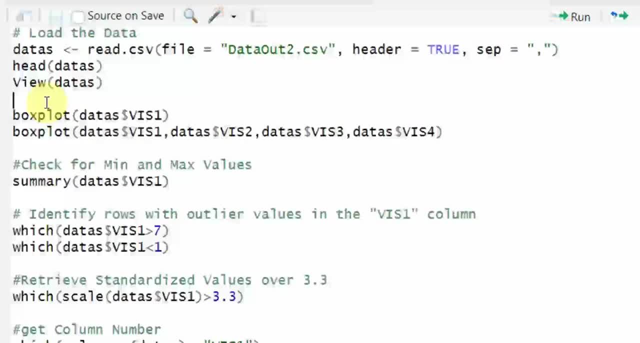 ones now, since we are interested in outliers again. the first thing that you can do is you can check for minimum and maximum values now. to do so, we need the summary function, and when there is a function, there are parentheses, and in this case, the argument is the data. 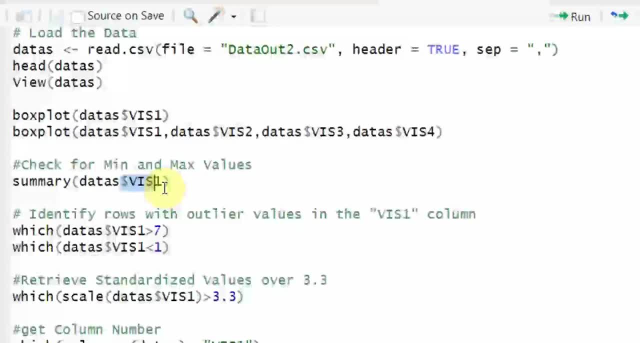 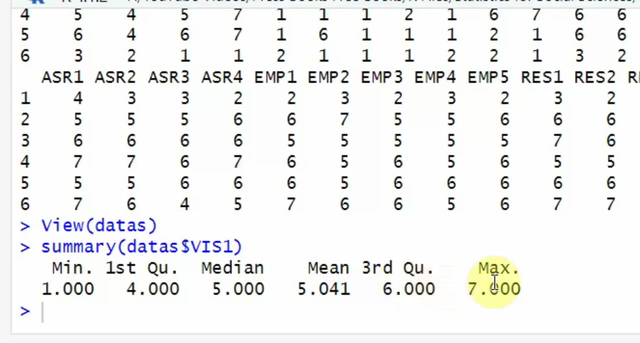 set that holds the data and the variable we are interested in. now. the data object is separated by a dollar sign from the variable name. so let's run it. the minimum value is one, the maximum value is 7, so there is no issue in the data set. but let's say, let me slightly change the 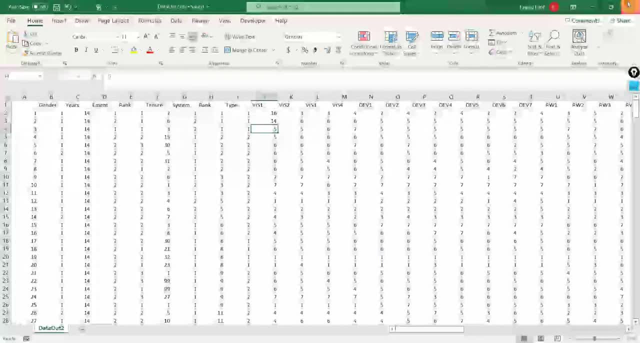 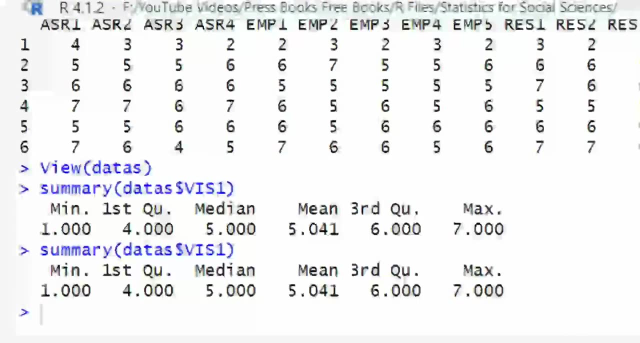 data. now that I have changed the data, let's run it now. look at this: the minimum value is 1. okay, now, although we have changed it, we haven't reloaded the data, so just make sure you reload it then. and now let's look at the summary. 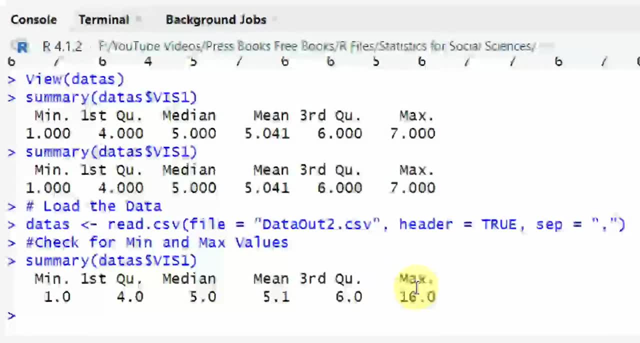 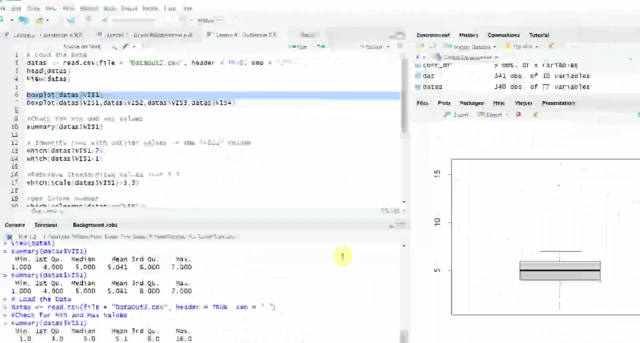 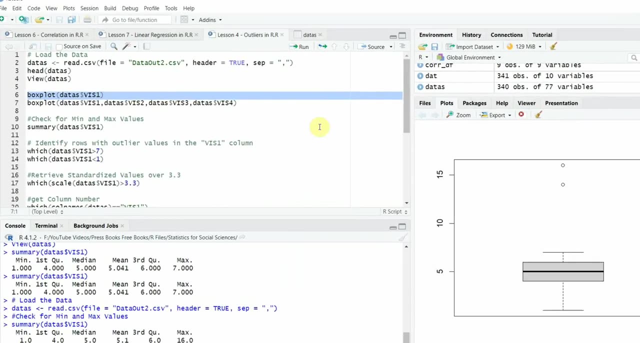 now it is done: maximum 16. now where is this 16? what observation or what are the observations that are causing this problem? so look at this. there are two observations in miss, in vision 1. now I do not know which ones are these, so I will find out. but first look at this. this is for a single variable box, not 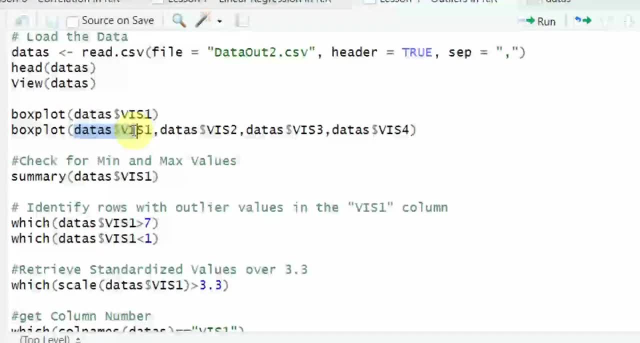 for single really variable. but if you've got more than one variable, again data, that is the object holding the data, dollar sign, then the variable name or the column name that you've got in your data file comma. the second variable comma on the third variable comma. on the fourth. 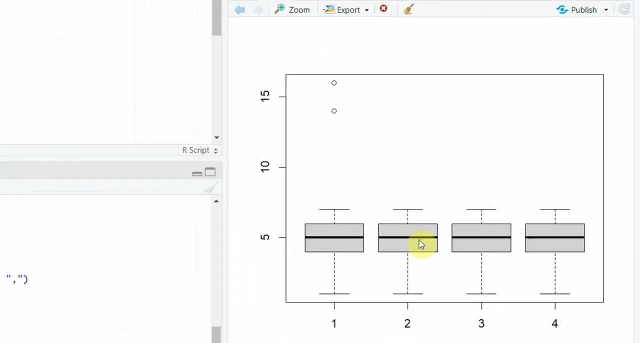 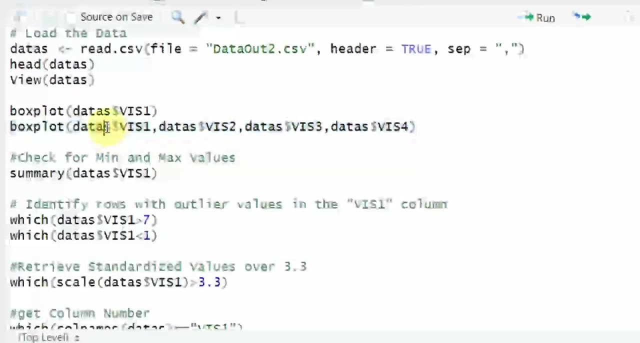 variable and when you run it, by selecting it, you will have all these four variables. now, these are the two observations that are outliers for the first one and which is the first one. vision is the first one. now, where or which observations are outliers? now, that's very easy you are going to use. 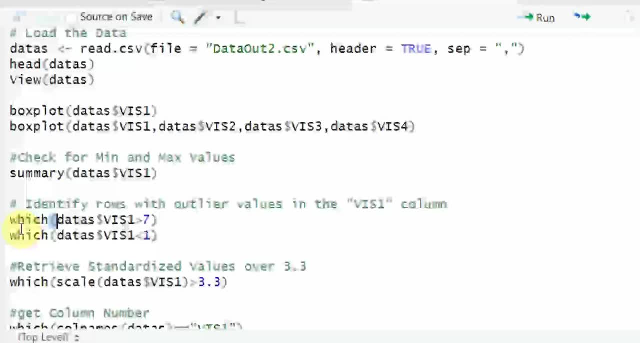 the which function, which parenthesis open. now when vision one, that is, vi s, variable one, the range is one to seven. now any value over seven is an outlier. so I'm just going to call which function. this is my variable in the data set, data s, and then the value greater than seven is an outlier. now which values are. 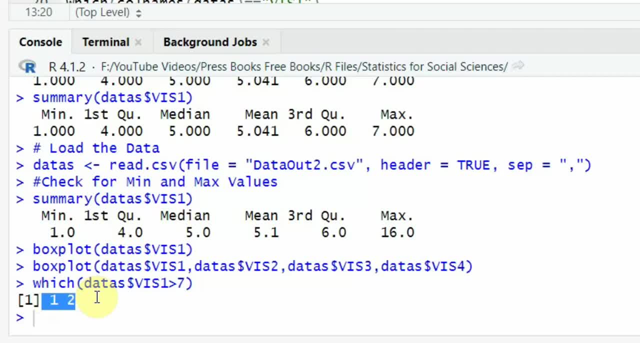 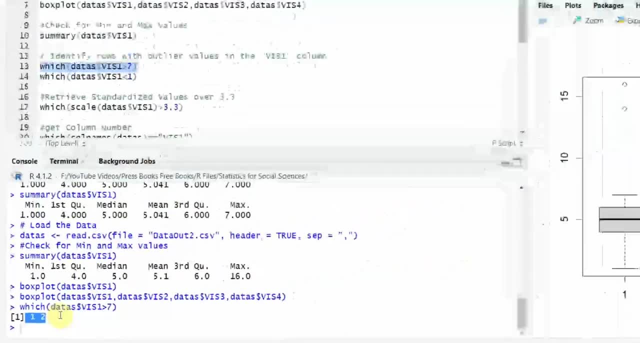 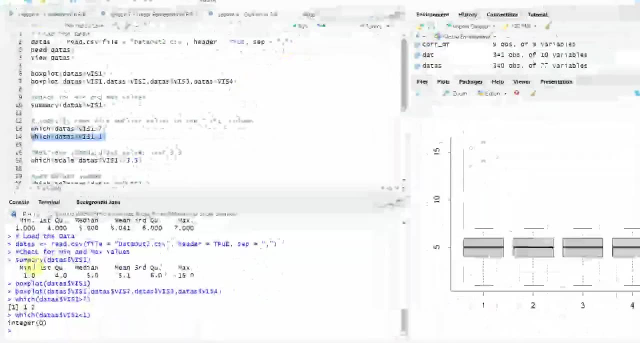 greater than seven. now, two values are greater than seven. response number one has got a value greater than seven and response number two has got a value greater than seven. for vision one: are there any values less than one? let's have a look. no, none of the values are less than one. now, as we 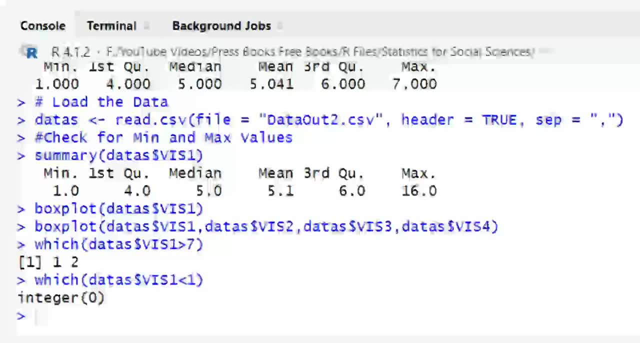 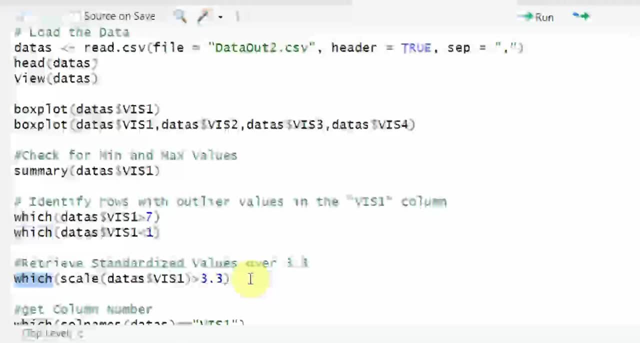 mentioned earlier, you can use a standardized score to find out the outliers as well. now, to do so again, I need which observations. have got a higher standardized score now. do you also need to have a standardized score now? do you need to have a standardized score? because in the case of which one is 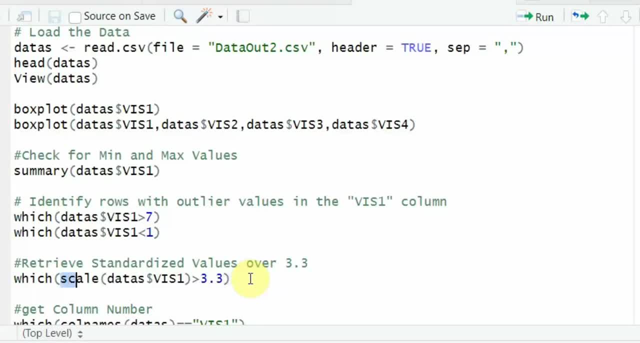 to get standardized score in r you need scale function. now scale function will be applied on a column in the data set that is data s object and that has got variable vision 1 and the value is greater than 3.3. now again, which observations has got greater than 3.33? z score 1 and 2 just. 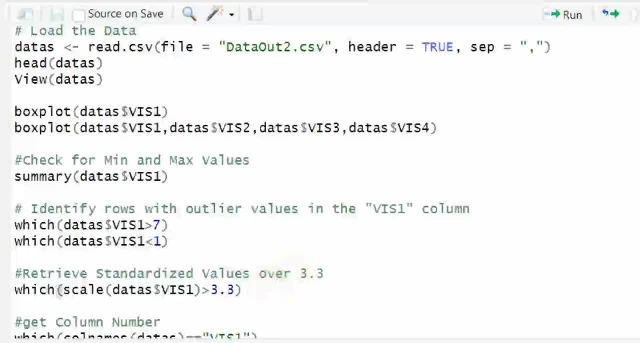 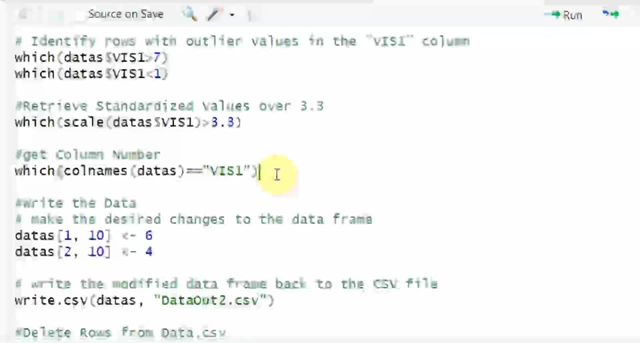 remember the parenthesis, how they are now. once you get this, now i know. okay, these are two. observation now: what is the column number for vision 1 so i can change the values? so to get the column number again, we are going to use which column name is equal to vision 1. so if this is the 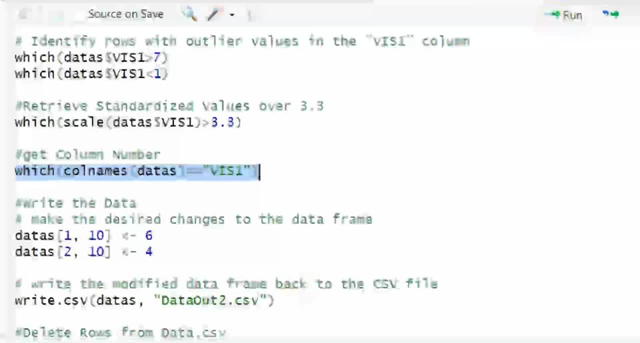 column name. get me the column number, and the column number is 10. now i know observation number 1 and this is observation number 1. this is observation number 2. now these are the two observations that are incorrect. so let's assume i've got some data at the back or i've got the 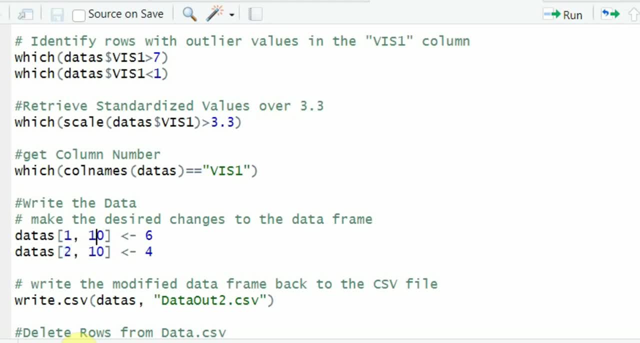 questionnaire in hard form. now, when i open the questionnaires, i found out that the observation 1 was not 16, but rather it was 6. the observation 2 was not 14, but rather it was 4, so data s is the object holding. my data observation is number 1. 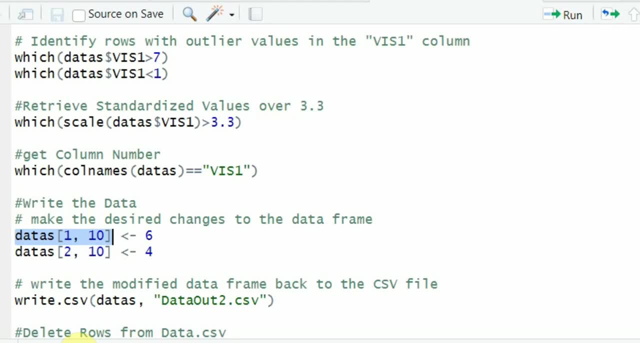 the column is number 10. look at the square brackets, these are not parenthesis- and the new value, or the correct value, is 6.. similarly, data object observation number 2, column number 10, and the value is 4.. now, once you change the values, you have to write the results back to the file. 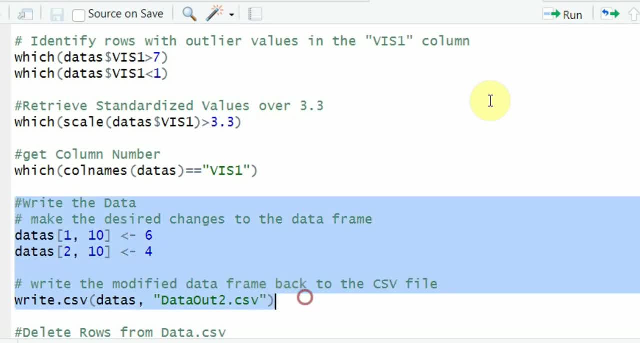 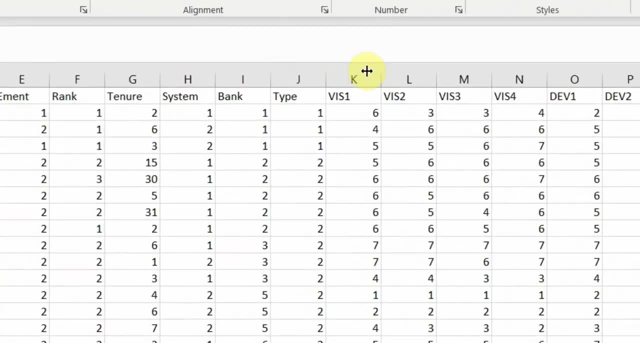 and once you do this, let's see what happens. run now, open the file and you'll see the changes. now look at this and you can see that the data object is now 16 and 4 rather than 16 and 4. the changes have been. 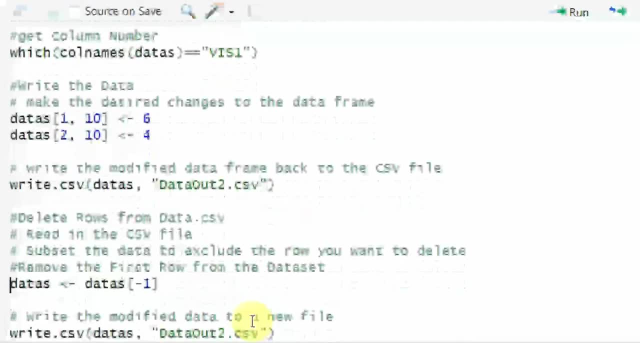 made. if you want to delete a particular row from the data again. let's say, data s is the object and i want to delete row number 1. so, similarly, just run it and you will be able to delete it. let's run it and now it is deleted again. do write the results back to the file after deletion or adding. 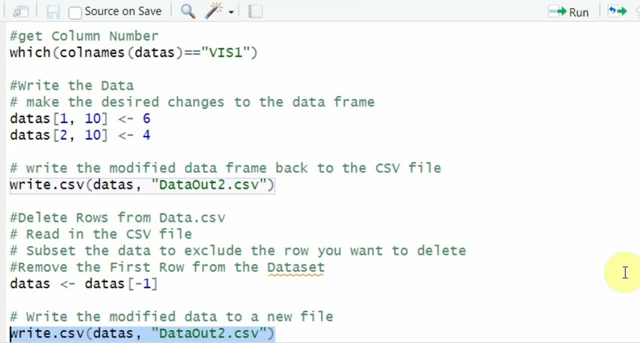 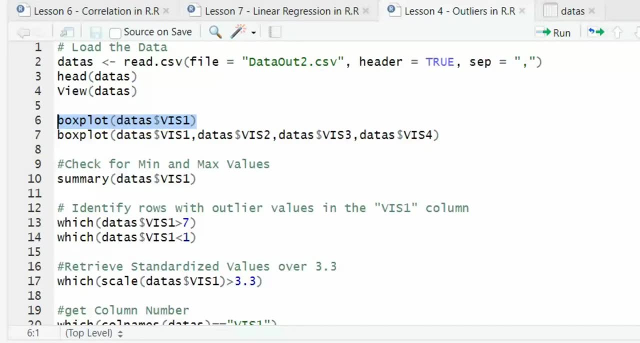 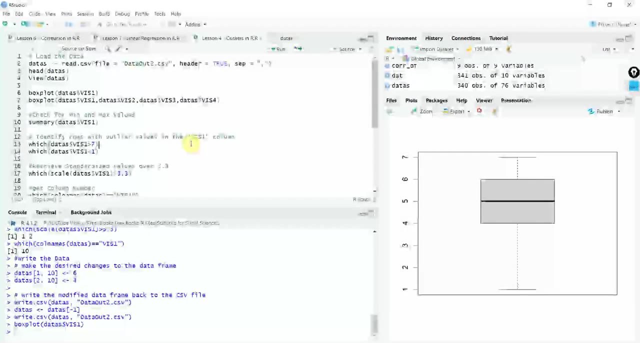 it to. the file is obviously ready. the results have been added back now. let's see. look at this. let's do this again. run and there are no outliers now, so this is how you can use r to assess your outliers. thank you very much.